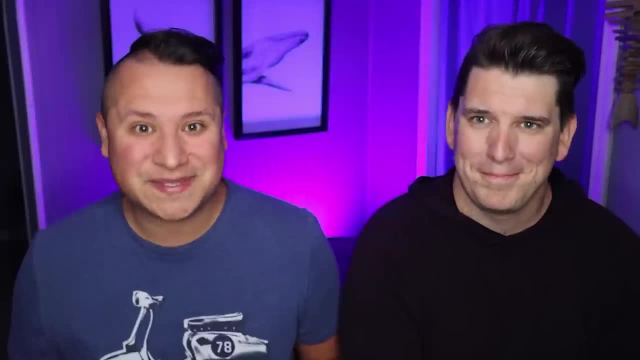 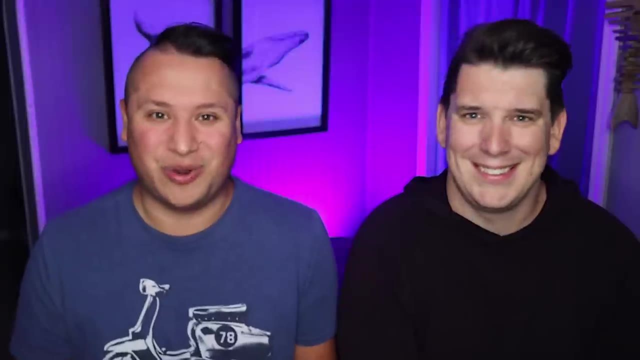 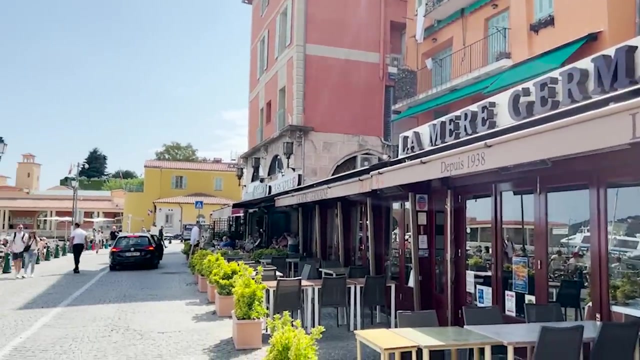 Within these, we're going to tell you the top Mediterranean cruise tips, Mediterranean cruise reviews, as well as the Mediterranean cruise excursion tips which we all know everyone wants to know. Now, many of you at home may have never cruised the Mediterranean, So today, in this Mediterranean cruise review, we hope to answer a lot of questions. 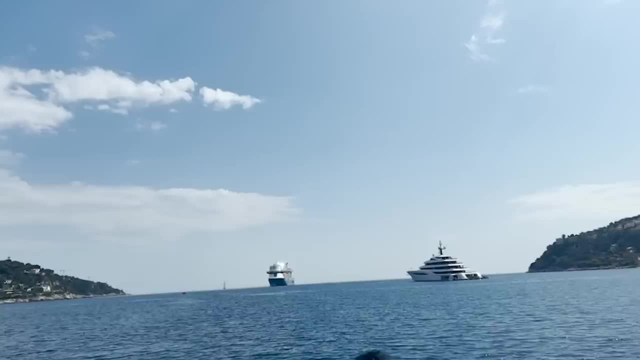 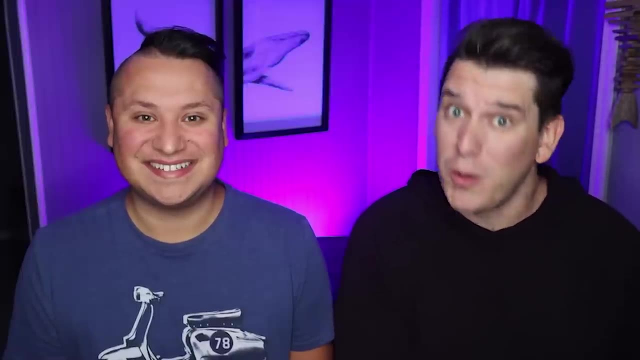 about excursions, what it's like to be on the ship, and talk about what it's actually like to sail in the Mediterranean Sea, Because we have found that it's quite different from sailing in the Caribbean. Let's get into the good, and of course we're going to talk about the bad, and then the ugly at the very. 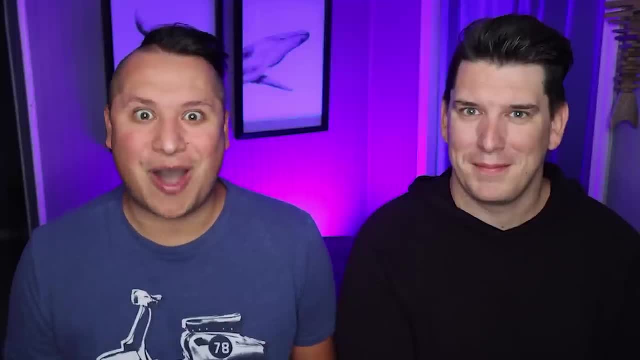 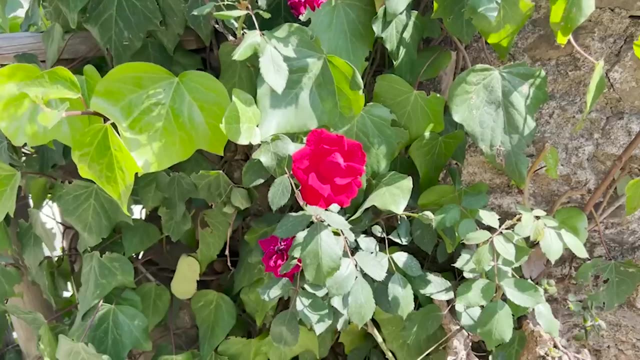 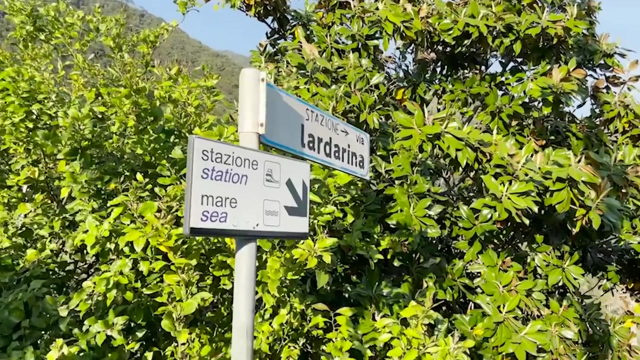 end. But let's start with the good, and first is the amount of ports, And not just any ports, new ports, I mean. you're going to new destinations, new countries every other day. There's rarely a day that you have just a normal sea day where you're just relaxing in the sun. No, you are on the go. 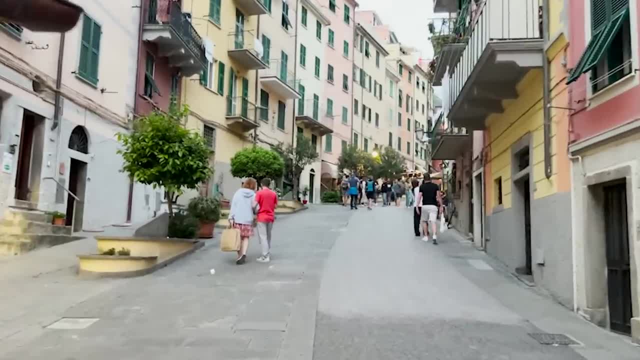 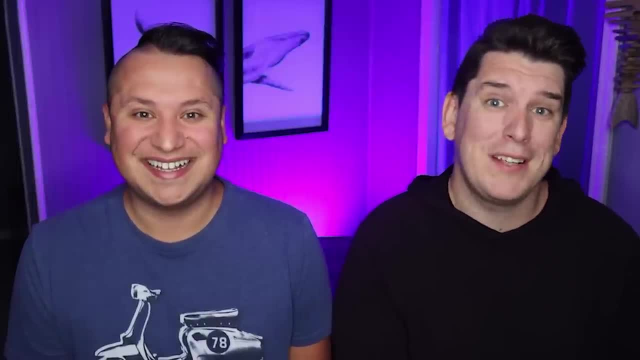 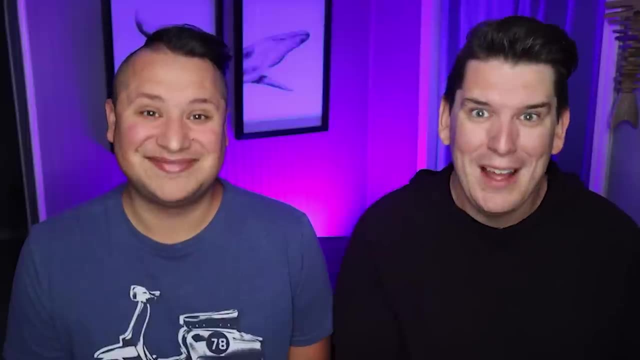 all the time figuring out different new cultures and really fun things to do while at port. Now we are sailing in the Mediterranean, actually twice, Once on the Celebrity Edge and once on the Celebrity Beyond, And between both ships we hit up around 13 ports in total over the period of two weeks. 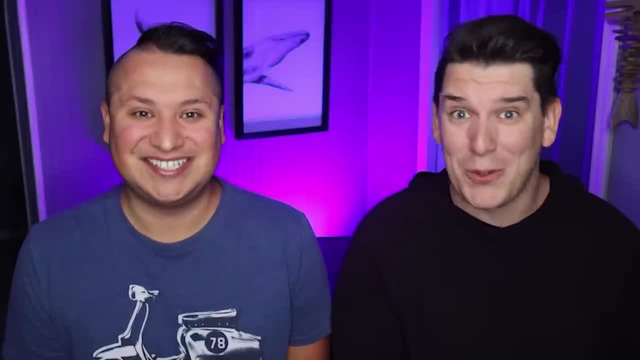 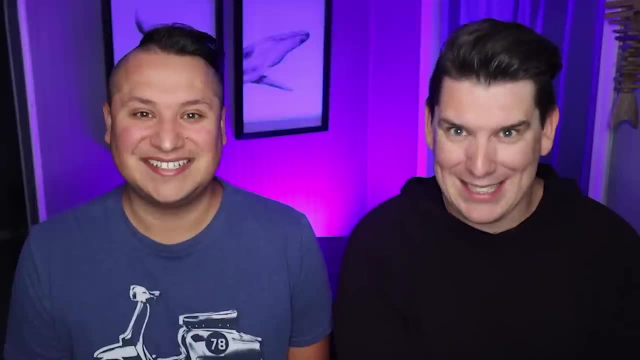 So that can tell you right there that there really wasn't many sea days on these cruises. It was great because these were ports we've not been to before In the Caribbean. we've been to Nassau and Cozumel many, many, many times, But it was really a once in a lifetime opportunity to get to go to places like 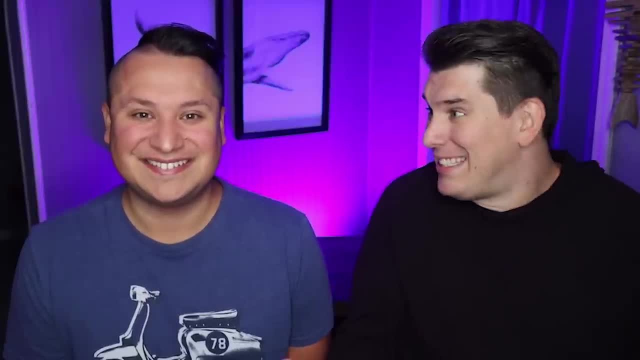 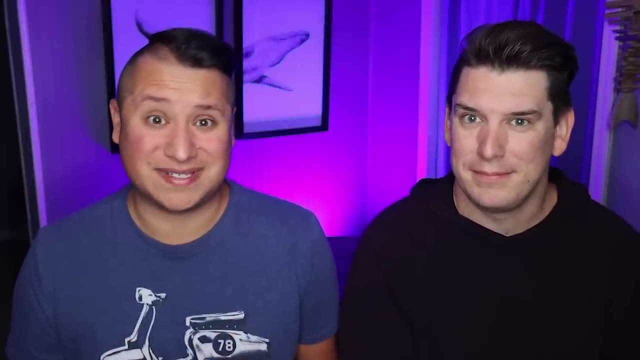 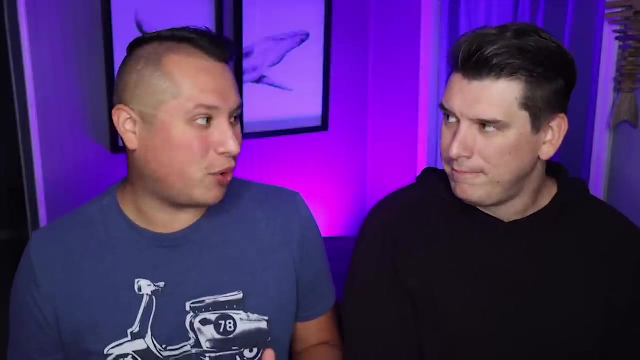 Italy, Monaco, Spain, France, I mean, we just we were all over the place and it was really really cool. Another great thing about this is that they were longer port stays as well. Not just more port stays, but longer days, Since we didn't have a long distance to travel. a lot of these ports were. 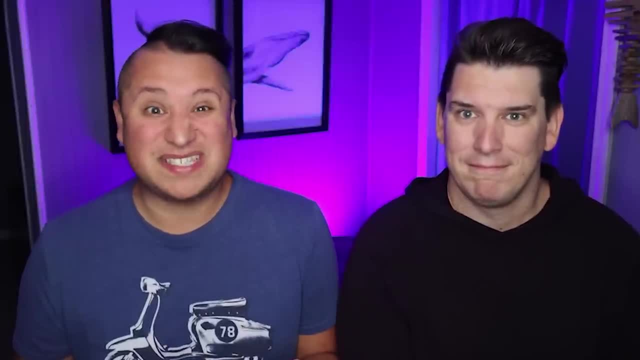 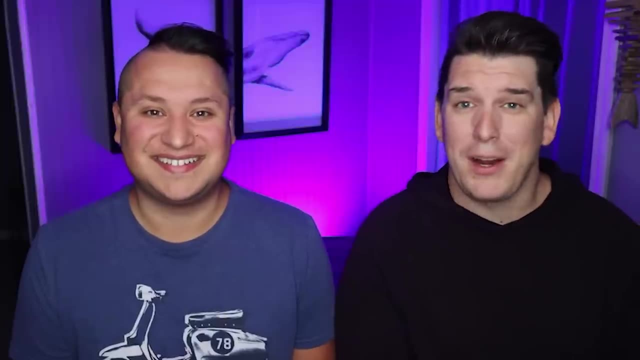 pretty close to each other. That meant that we got up at maybe 7 or 8 am in the morning, got off and came back sometimes when it was dark out outside. Now, because the ports in the Mediterranean and you're not going long distances, you're typically traveling at a very slow speed. 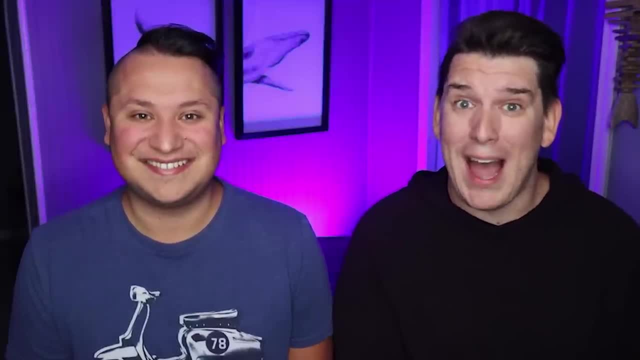 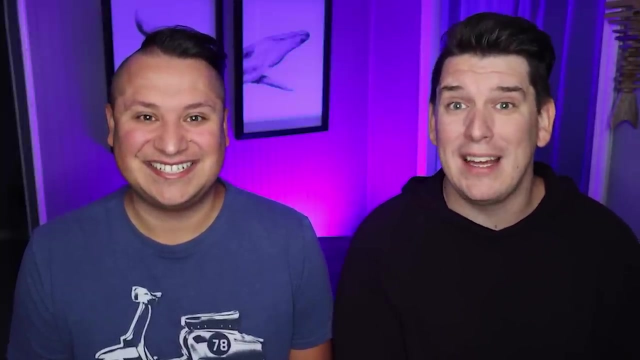 Now this is great, because rarely do you actually feel the motion in the ocean. A lot of people do experience seasickness and getting a little queasy, especially when the waters can get choppy. The Mediterranean Sea, for the most part for the two weeks while we were sailing. 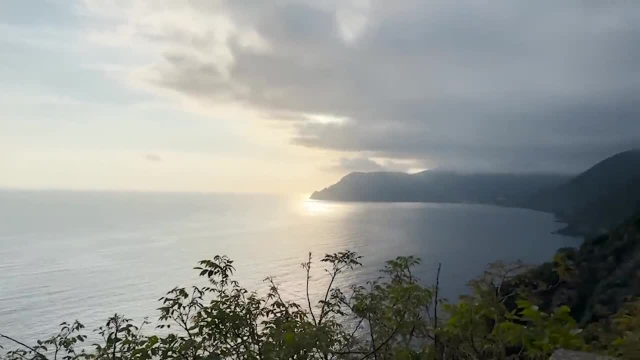 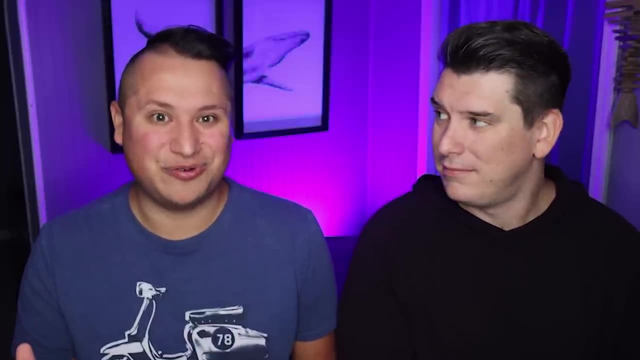 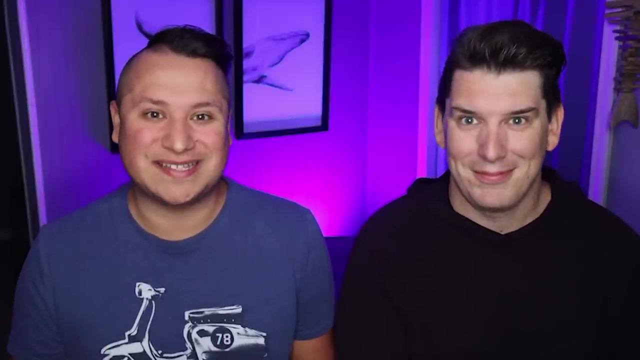 was very calm and rarely do I remember actually feeling the ship rock at all. Many times at during dinner we actually looked out from the main dining room on board the ship and could just see it almost looked like glass because it was so smooth. It was truly an awesome experience and 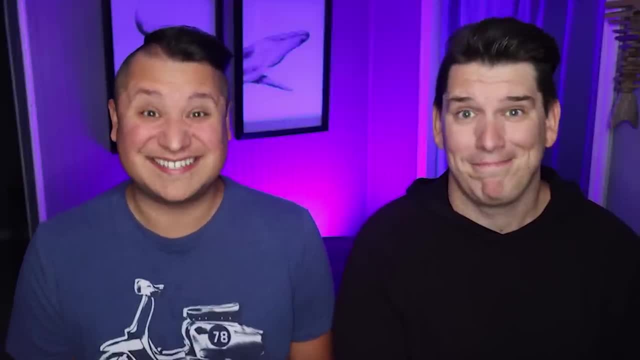 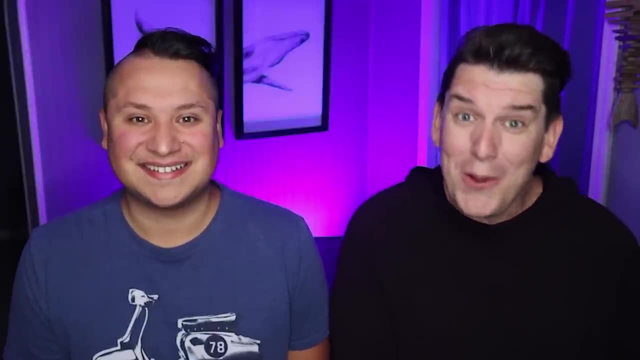 really a good place to go if you're someone who's prone to seasickness. Now, not only do you get diversity in the people that you're around and the cultures that you're experiencing at port, you also get that on the ships, And this is very different from cruising in North America, where 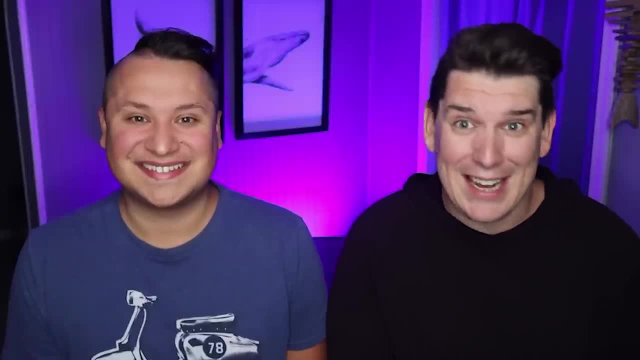 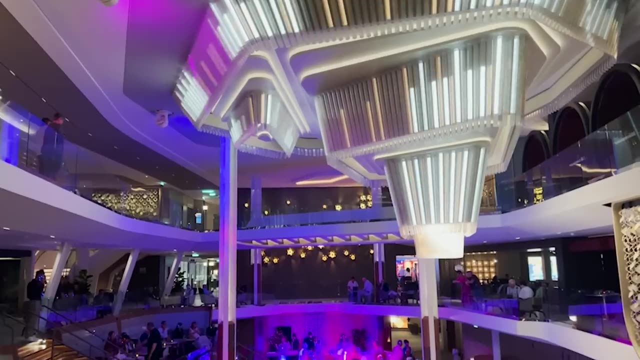 primarily, many of the guests are from the United States and Canada. When you're in Europe, you have people that are truly from all over the world. I think on our cruise we met people from throughout Europe, from Australia. It was a very, very cool experience to 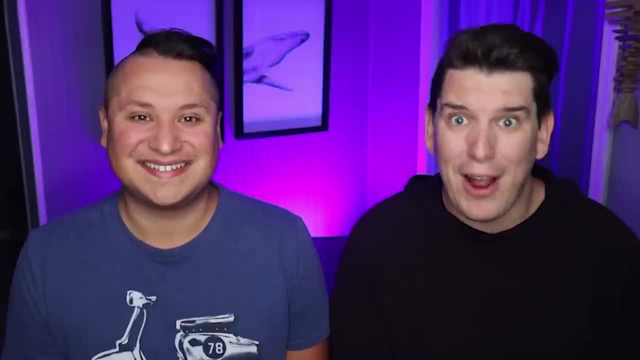 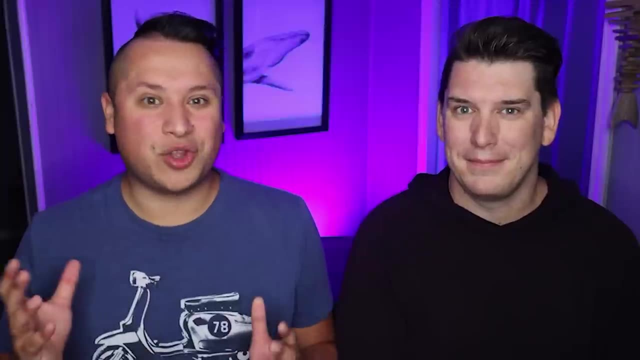 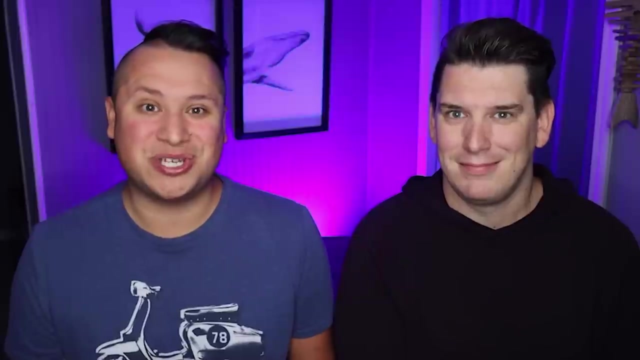 get to mingle and meet with other travelers from different backgrounds and different countries, because you don't often get that when you're sailing from North America. I think one of the coolest parts for me is just seeing the amount of different languages spoken, Of course, on board this ship, since it was a celebrity ship. 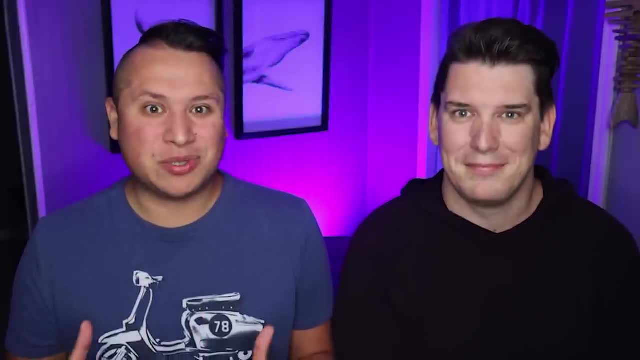 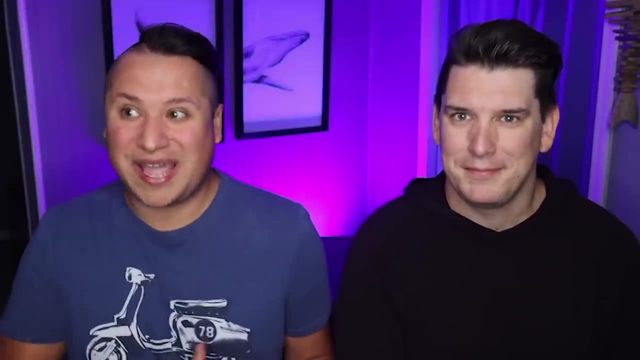 English was the number one spoken language, but it was almost the communal language. There was still a lot of people that spoke all the different native languages, from whatever countries they came from, and you got to go ahead and witness that at port as well. It was just a really cool. 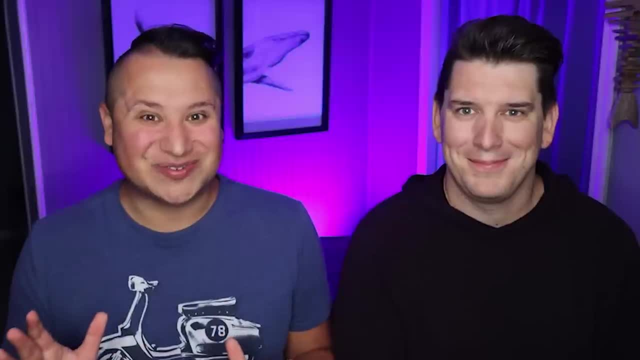 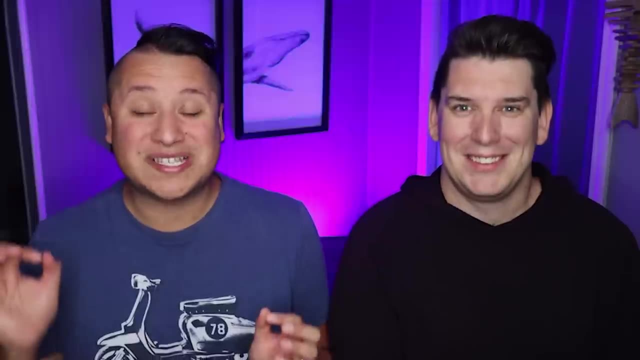 thing that we don't get a lot of back in the States. This next one, I am sure you all are ready for It, is the food while at port. The food at port was phenomenal, and a tip here for MedTrain cruises: MedTrain cruise tip. 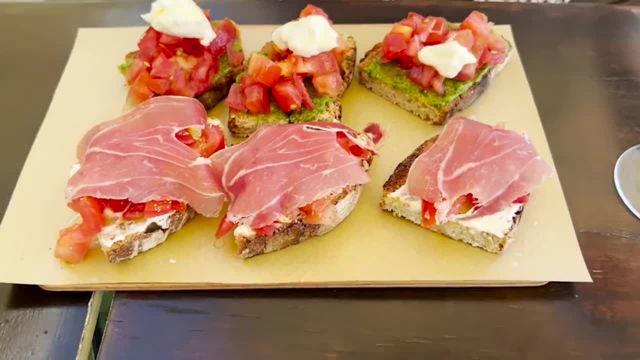 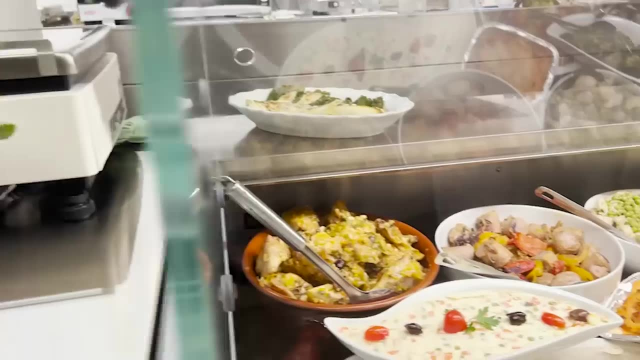 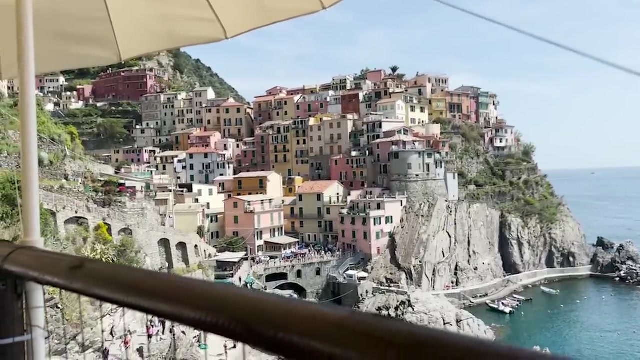 would be that you have to use some kind of trip advisor or some kind of online tool to find those best hidden spots, because when you find those local gems, oh my gosh, your mouth will salivate just wanting it over and over again. Now, this is a place where you're going to want to plan and 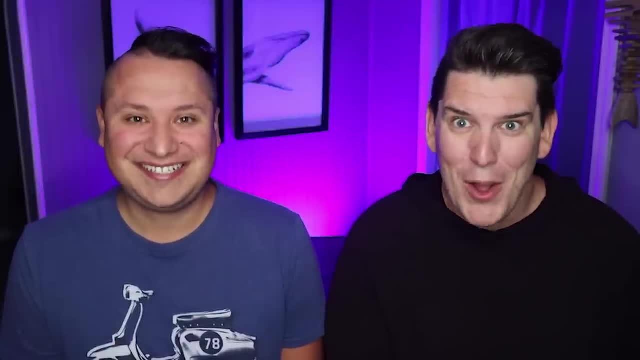 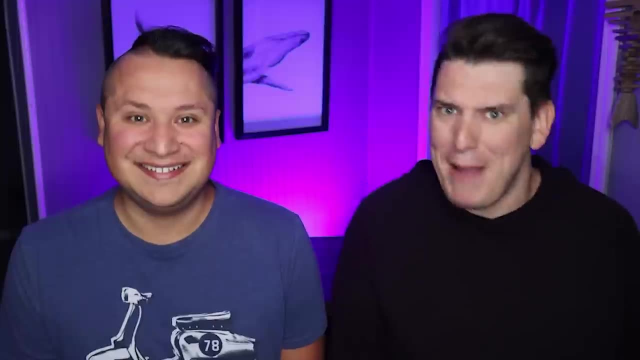 budget a little bit for money that you're spending off of the ship Rarely. when we're cruising in the Caribbean, do we make sure that we're going to have lunch and dinner off the ship? because we've already done that, of course, But when you're in Europe and Italy and you have access to freshly made 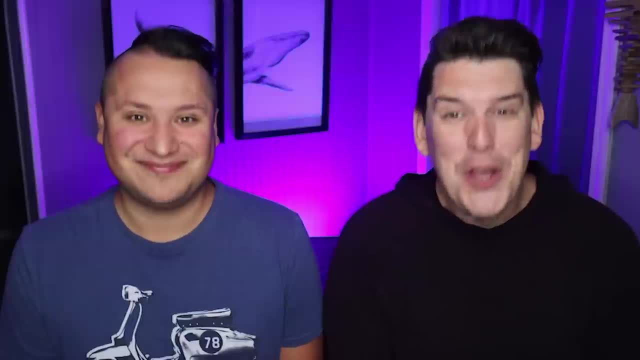 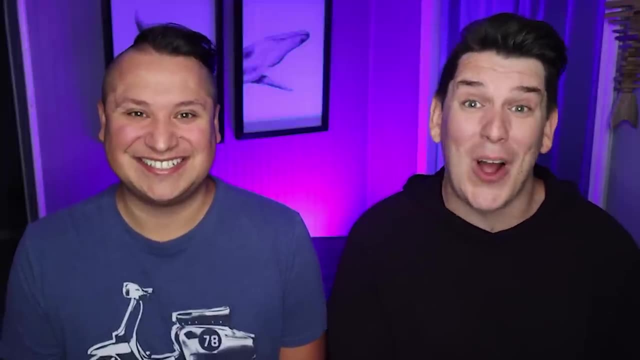 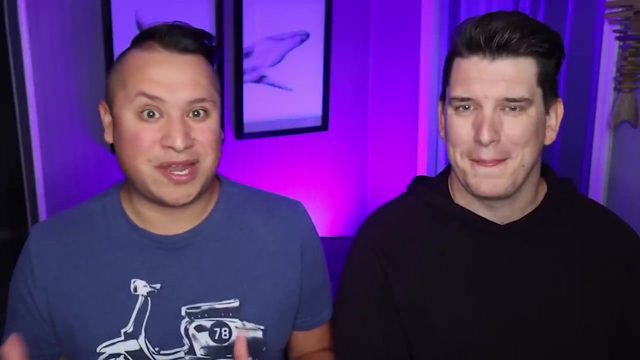 pastas and pizzas and food that you can only get there. you better believe that we're not eating on the ship and we are eating at every single port whenever we get the chance to, and we were not sorry that we did it. The food was wow. Now, if you're new to Mediterranean cruising and never been over to any parts of Europe. most countries in Europe are a part of the EU- the same currency called the euro. the good thing about this is that you can kind of take out a good lump sum and use it at every single port and not have to change it up per port. 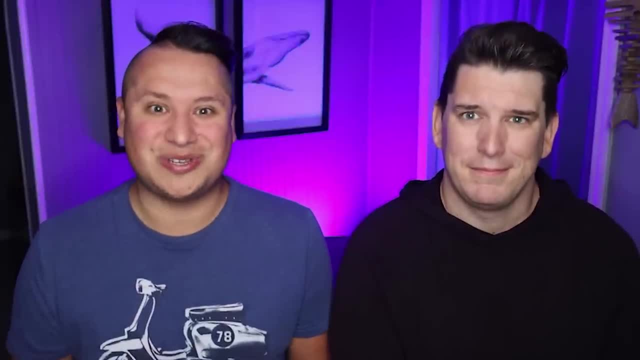 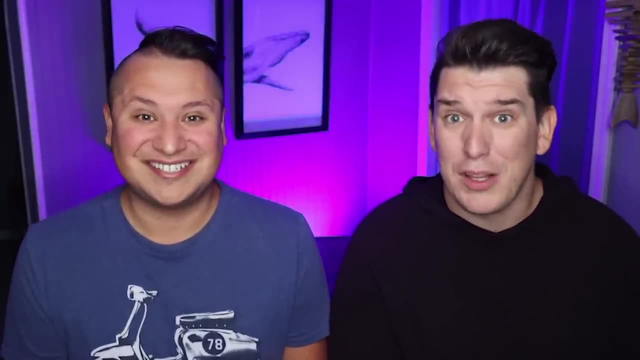 something very basic, but if you've never gone, we just want to make sure that you know that that is a kind of a good plus for Mediterranean cruising. If you get on a ship or you fly over there without the euro, you actually can exchange that money on board. that was something that we did multiple. 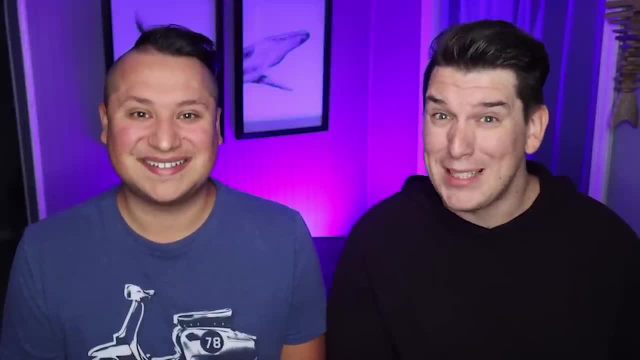 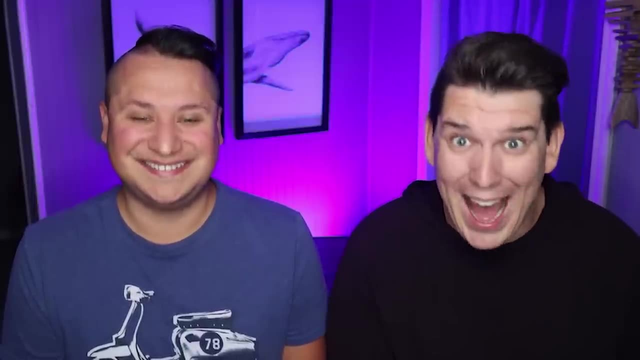 times down at the guest services desk and we actually found the rate to be pretty reasonable, especially when we had stopped in ports where the exchange rate would be dramatically high for the US dollar. of course they know the tourists are coming in every single day, so check that out. 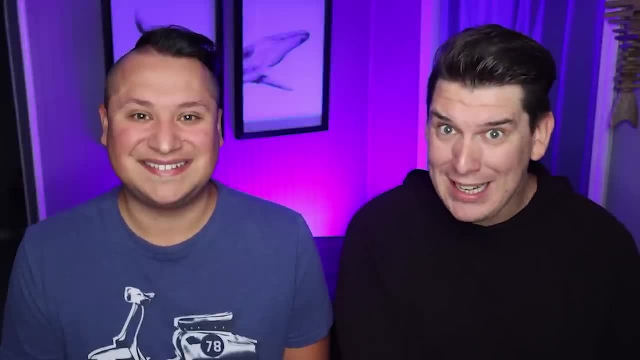 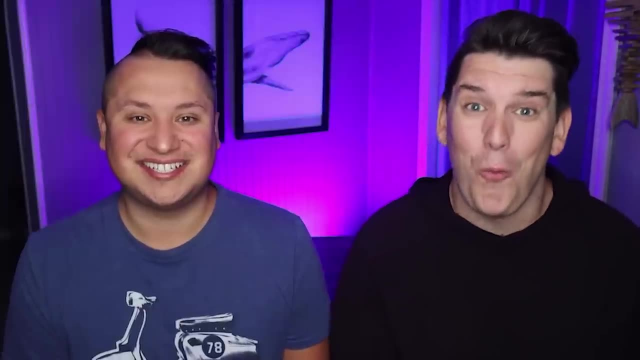 and find a good place before you go to the Mediterranean to exchange those dollars, so that you don't have to lose a lot of your money. One last thing here that we have to mention is the weather. Now we went in late April, early May and we were expecting cooler temperatures in the 50s. 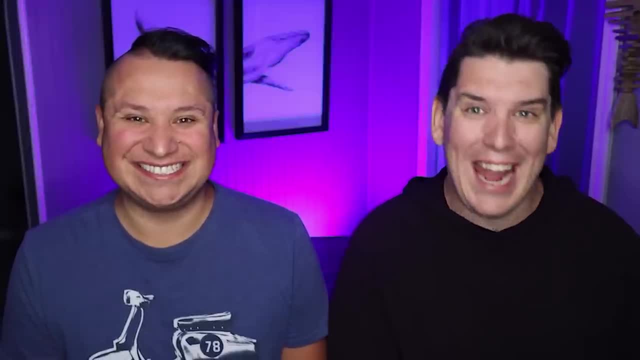 and 60s. That was not what we were expecting. We were expecting a little bit cooler temperatures in the 50s and 60s. What we got it was in the 80s and every day at port it was hot. Now it did get cooler in the evening. 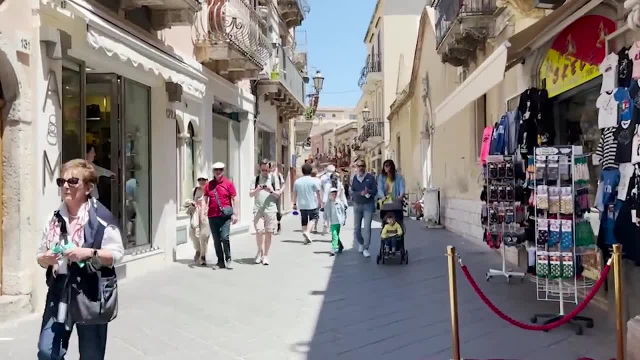 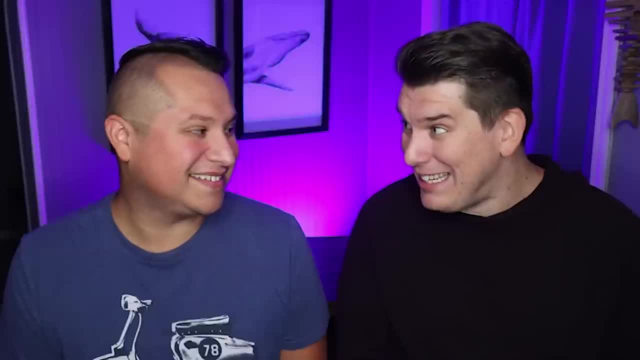 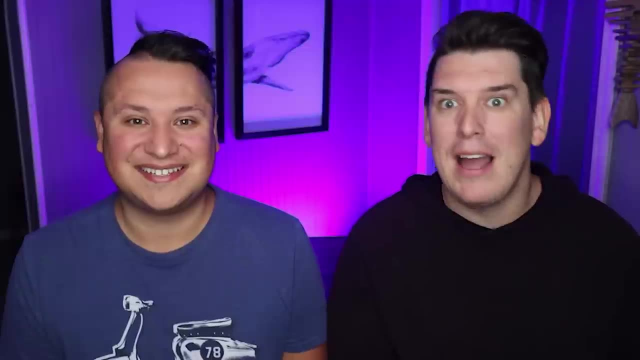 but you definitely want to pay attention to the weather when you're going over there. The Mediterranean weather can be quite volatile in terms of the temperature. It was a lot hotter than expected the weeks that we were there, but of course it's still springtime if you're going in April and it could be a bit cooler. So keep in mind. 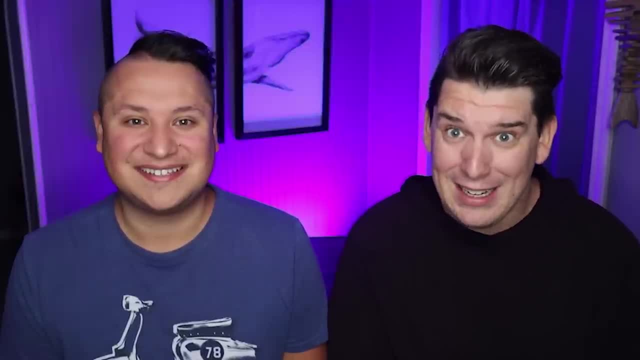 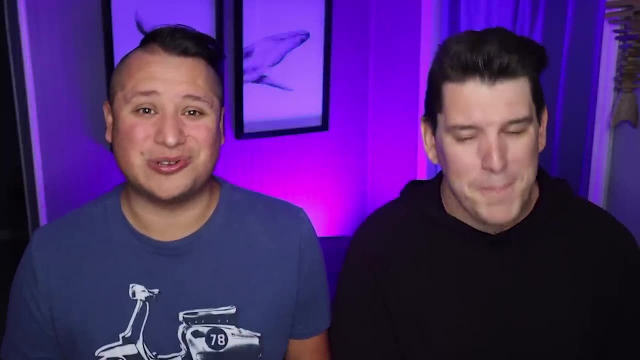 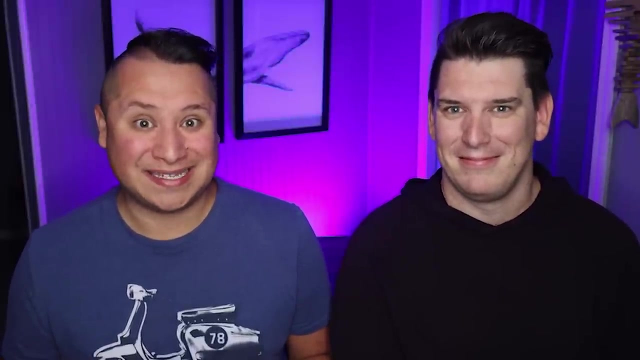 the weather is going to be different from the Mediterranean, but it may be hotter than expected. All right, that was a lot of good and we did have a fantastic Mediterranean cruise. so please take this next thing as more of FYI's of what were the bad experiences that we did not expect and had to. experience ourselves. The first bad is a lot of the big destinations you think of aren't necessarily close to port. This happened almost every single port we went to where, even like Rome, Italy, is not anywhere close to the port that you actually port in, and so you do have long distances for a transfer. 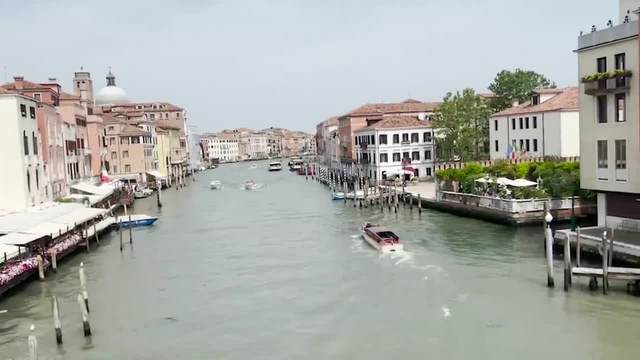 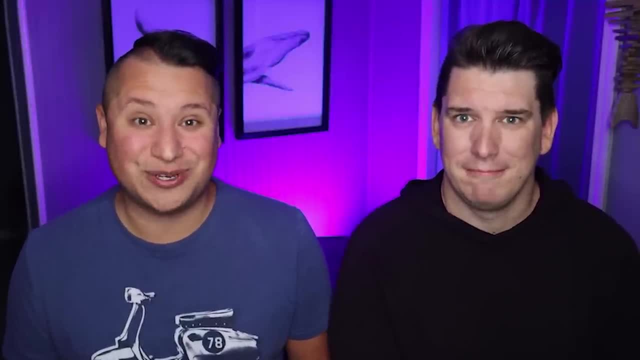 or some kind of transit that you have to pay- maybe an hour, two or three hours- to get to one of these huge destinations. it's part of the reason why you have to have long days when you're cruising the Mediterranean to hit these big, actual cities and destinations you want to go to. But it is 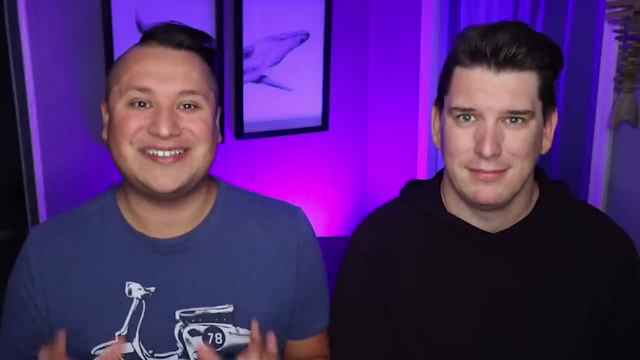 something just to note, not necessarily the worst thing ever, just something to note and be prepared for. Something else to note is the weather at the end of the year, and we'll get to that in just a moment. Let's talk about other situations, and if you're going to be going to the Mediterranean or other important times in the year, you might want to start off with the weather on the island or in other places. 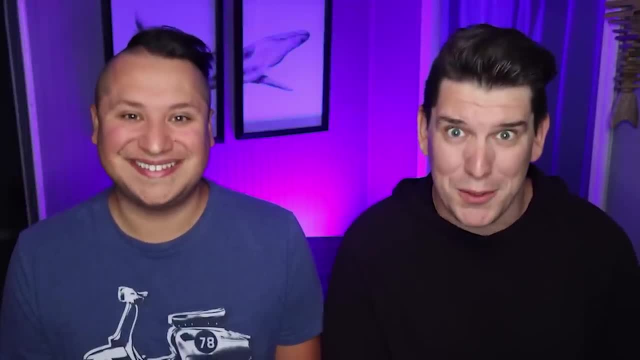 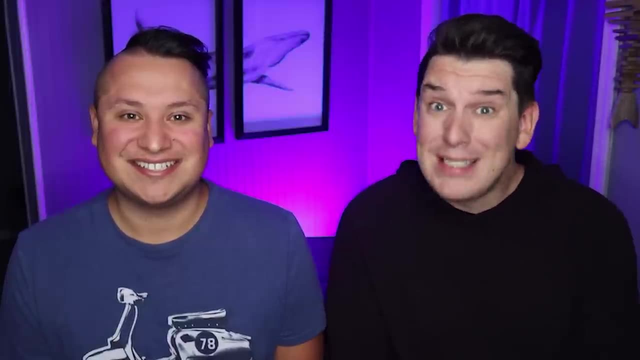 the food on board is going to be a little bit different than what you might be used to. Now you're in the Mediterranean, you're in Europe, so there was a lot less American food, especially in the buffet. There was a lot more seafood. Now, someone that does not love seafood- 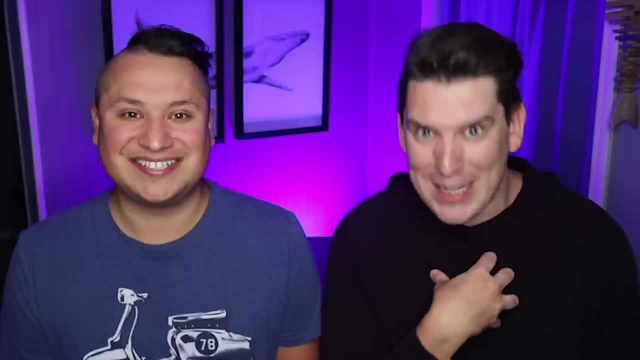 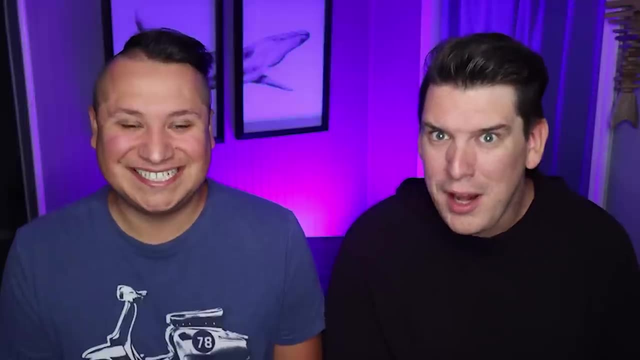 might have a little bit of a hard time finding stuff to eat. That would be myself. I'm not a big seafood person, so there would be times that I didn't find things that I loved on board. Um, but you save that appetite for when you get off the ship and you eat all the pasta you could. 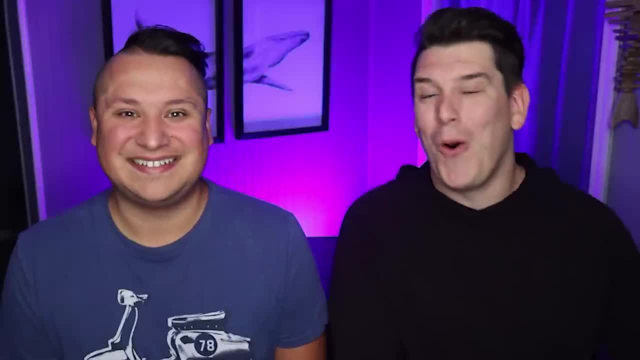 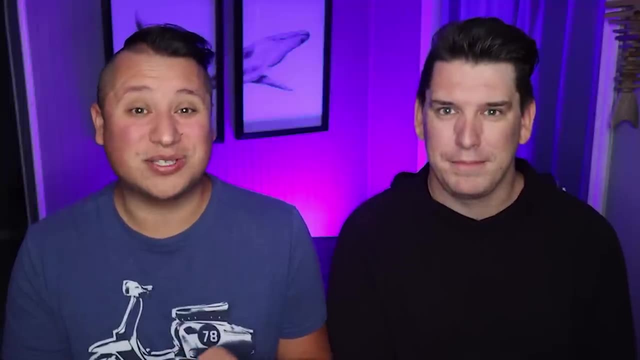 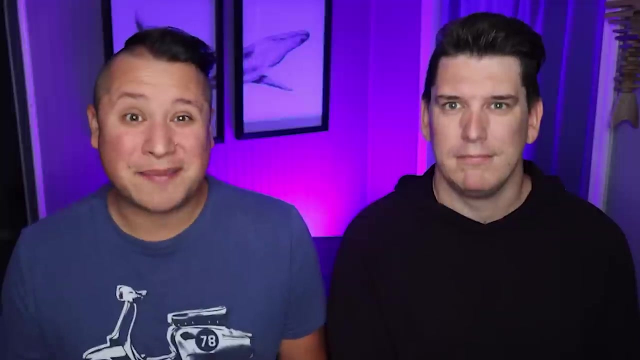 ever want, because I think there was pasta or tapas or a lot of different types of wonderful food on land. Yeah, one thing to note here is seafood is very common, but also like olives and lemons. These are some of the more natural produce and natural resources that they have in the Mediterranean. So of course the cruise lines are going to do what is more abundant and more resourceful And they're going to go and use those resources. So, just so you know, those are more of the types of Mediterranean cuisine. If those aren't your well favorites, you might not have the best food. 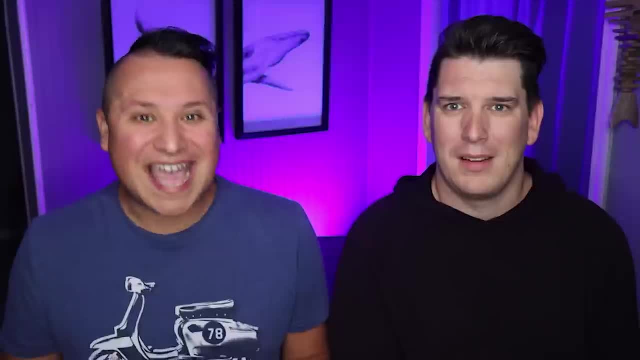 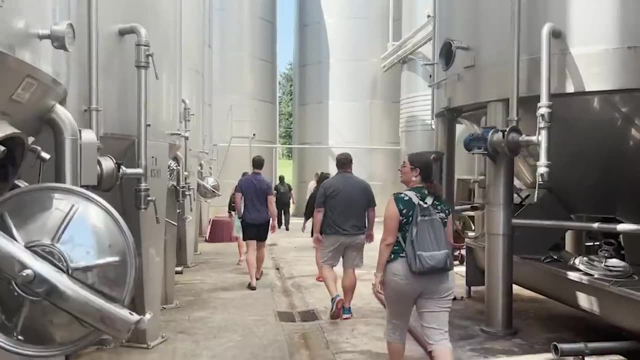 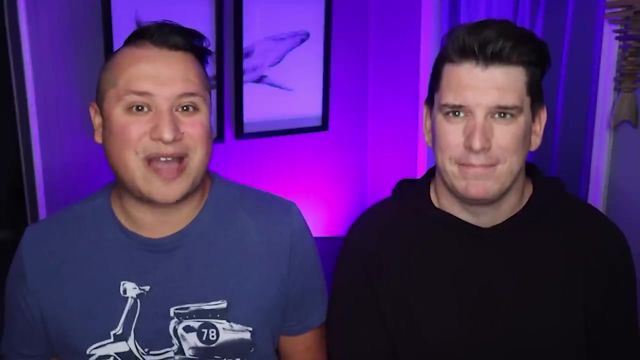 while on board, but you can get off at port and eat like kings. Next thing that we have to say that is bad, unfortunately, is the expensive excursions on Mediterranean cruises. As you know, Mediterranean cruises are already going to be a higher cost for anyone traveling. 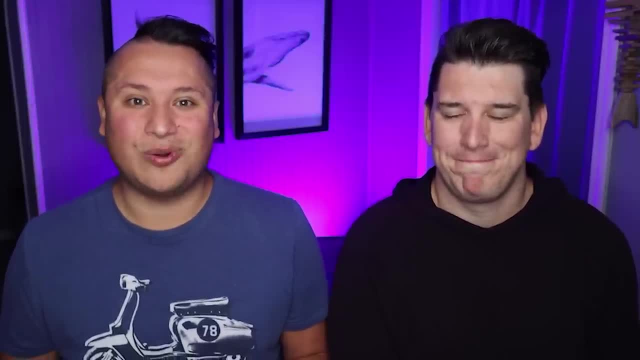 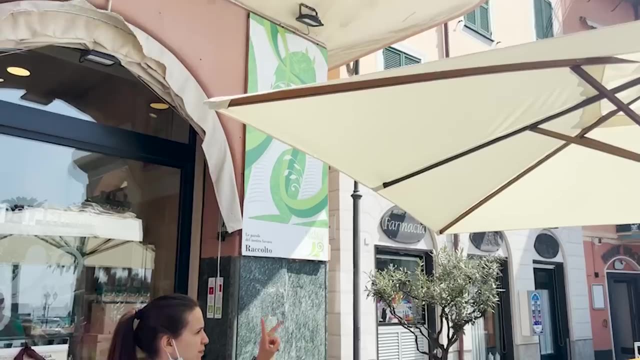 outside of Europe and in the Mediterranean. So when you get there you hope that you can do a lot of things at ports or for cheap. That is not the case. In fact, a lot of excursions are really expensive And if you just do a little bit of research you can usually do them much cheaper. 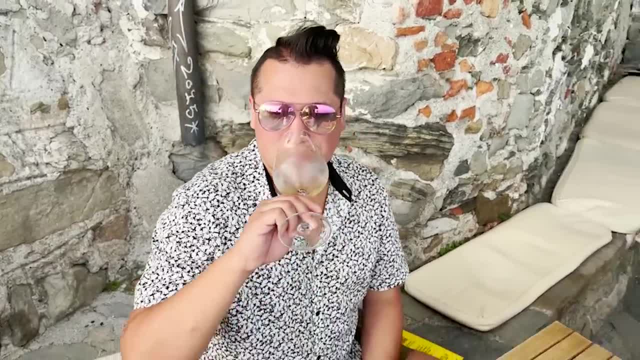 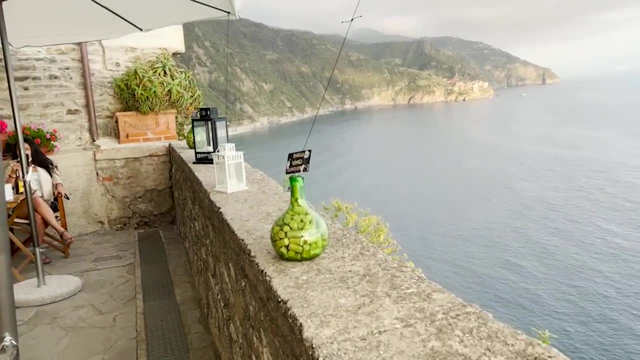 on your own. Taking the train or any other kind of public transit that's available is a lot of times cheaper, and something that just takes a little work and research but will get you a lot further with your dollar. Now, not only are the excursions more expensive, but they're also more. 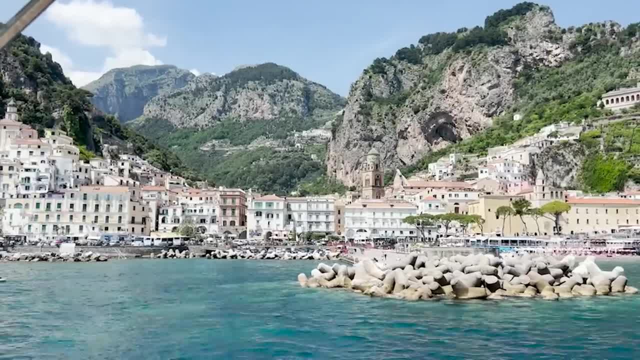 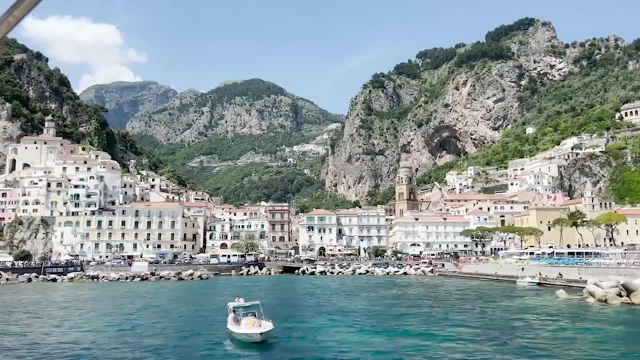 expensive. They also tend to be longer, And that's kind of going back to the point of most major destinations or points of interest are not right next to the port. You're going to want to listen to this tip because it's very important for your planning When you are planning excursions. 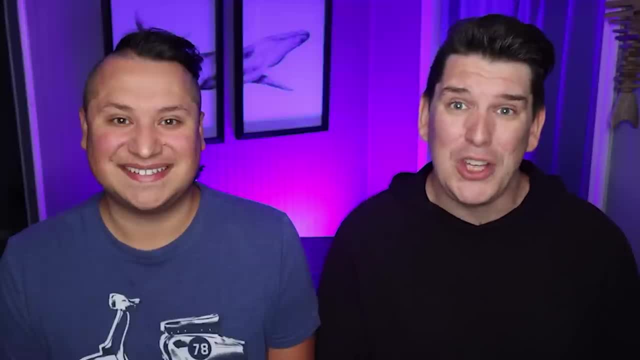 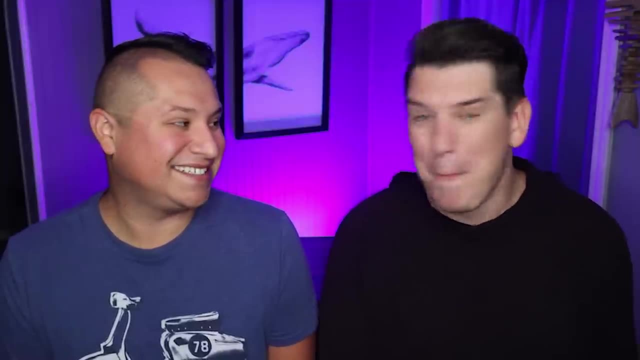 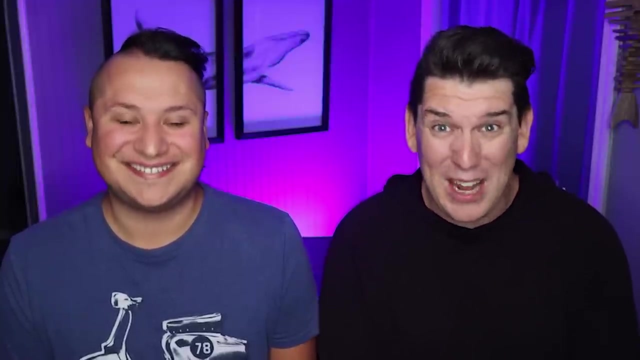 for your Mediterranean cruise. we do not recommend that you do two long excursions on back-to-back days. We did this and this was probably our biggest faux pas during our Mediterranean cruise. We woke up, we had a 10-hour excursion. we got back to the room pretty late. we were 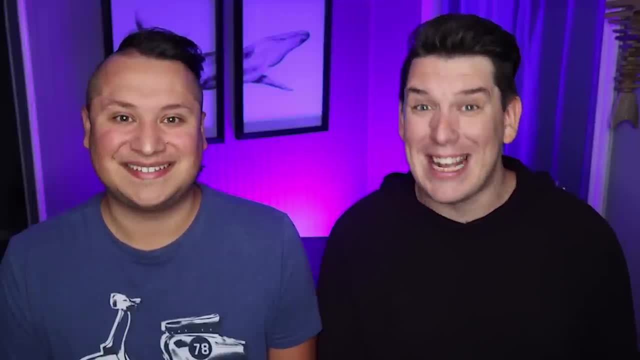 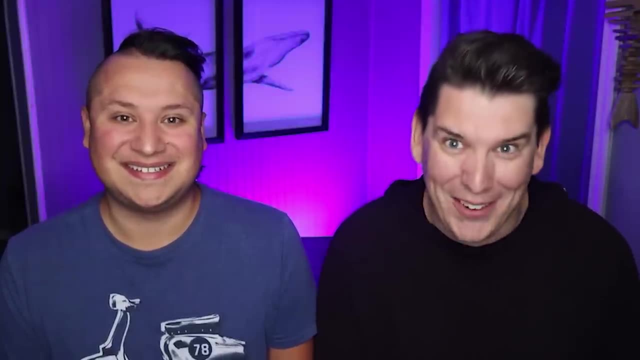 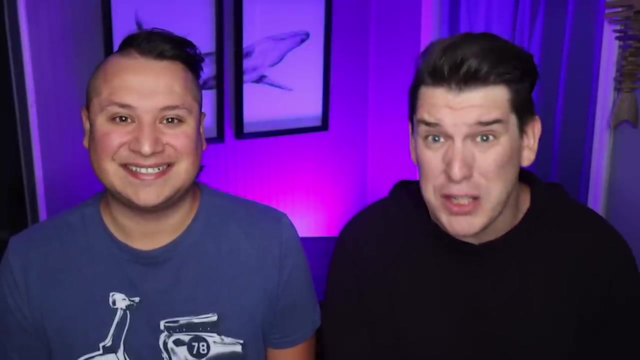 exhausted, and then we had to wake up at 6 am the next day for another 10-hour excursion. When you do this multiple days in a row, your body just eventually gives out, because you're traveling, you're walking a lot and these are super long days that you need a lot of energy for. So we 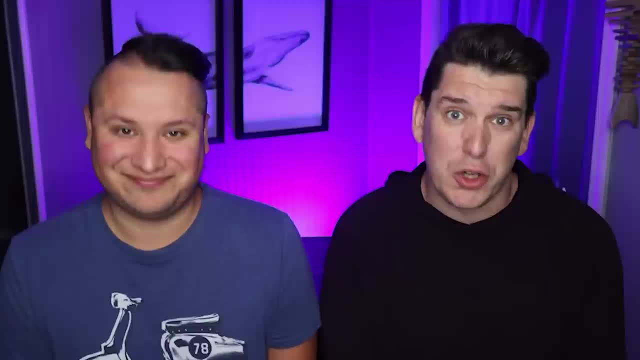 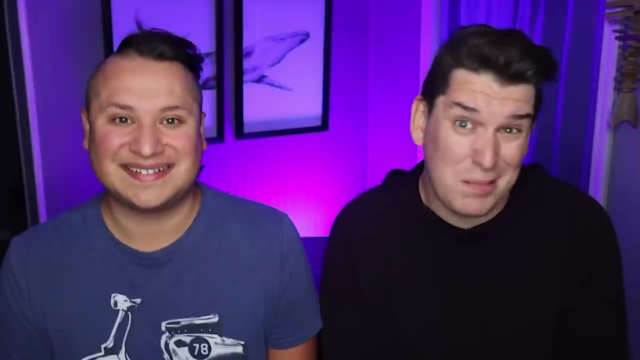 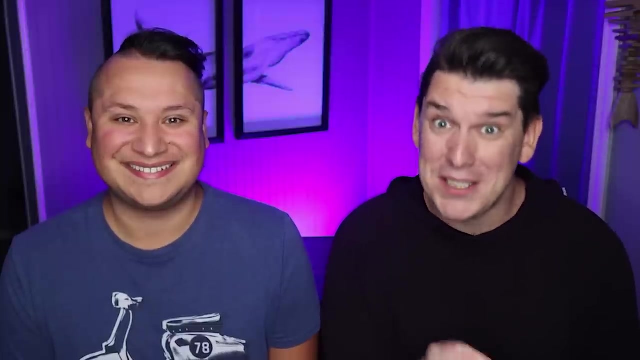 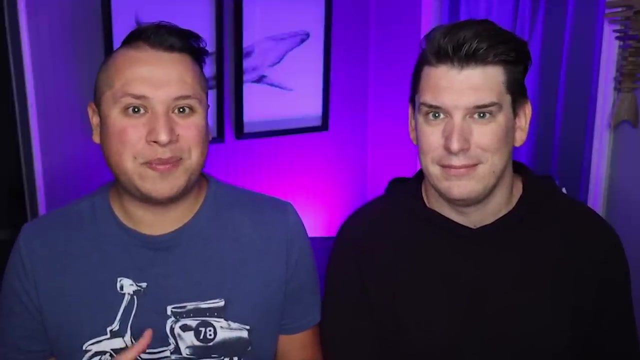 would definitely recommend giving yourself a break in between long excursions if you are going to hit up major destinations. This is something else that you just need to know while you're at port that a lot of times there will be a charge to use the restroom while at port. Once again, not bad, It's a cultural difference. 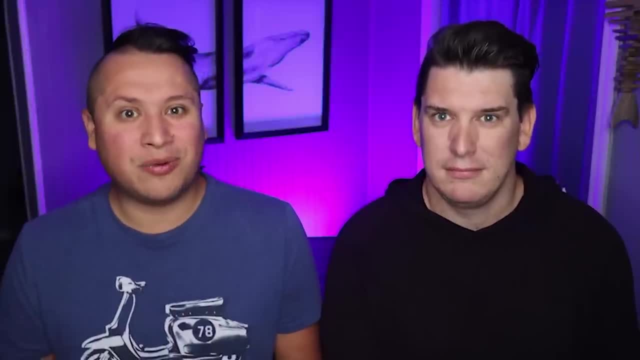 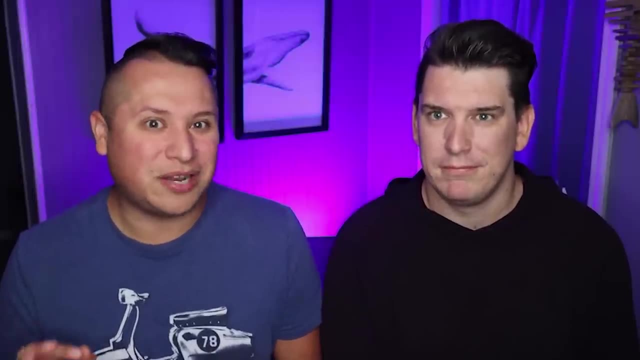 and something that we need to make you aware of. So bring along some very small euros- and this is, along with the currency thing, that you do really need to have just a little bit of euros on you at all times, because no one likes it not having the chance to use the restroom because you don't have. 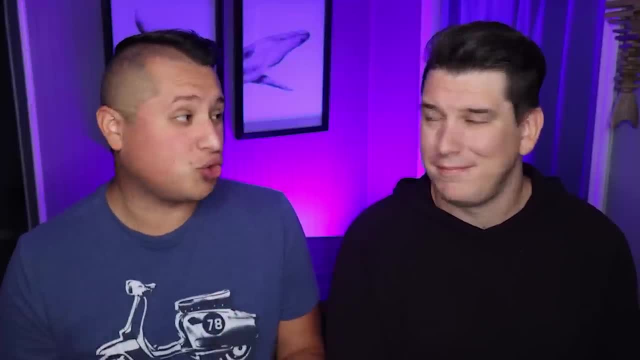 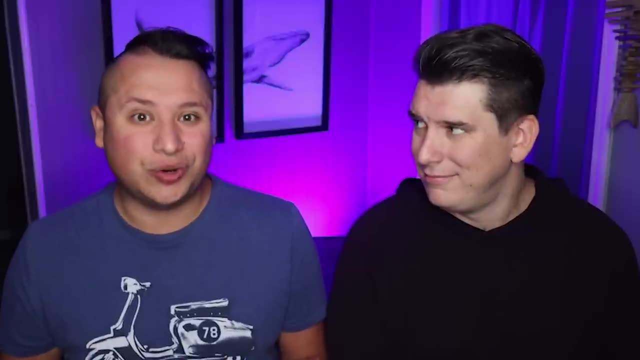 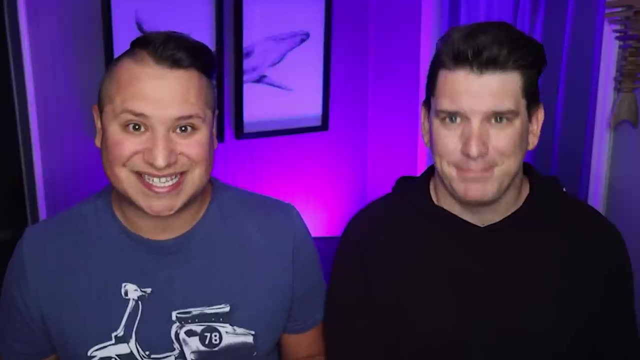 a euro on you. Now, this last one is a little complex, but it was a true rude awakening for a lot of people. So stick with me here. but there is a value-added tax in the EU for specific itineraries. Now what this value-added tax is for is for any onboard purchases. This can include 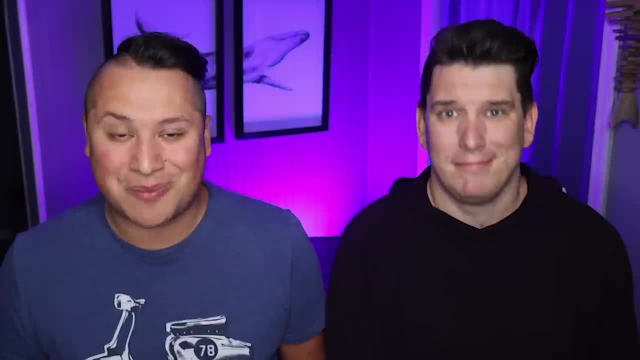 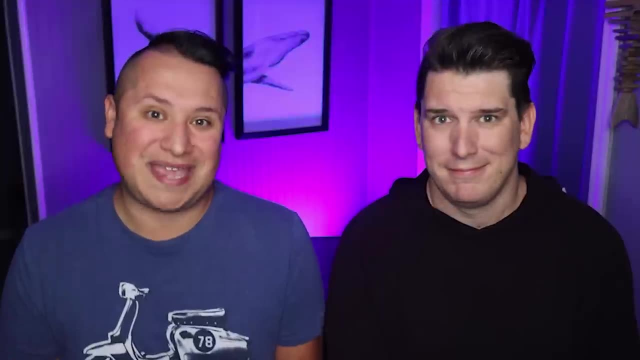 beverage packages, beverage package upgrades while onboard, as well as shopping onboard or other things that you do onboard. The big part of this is knowing when it can be added. If you are doing an itinerary with all EU ports, that means you have not a single destination. that is not a part. 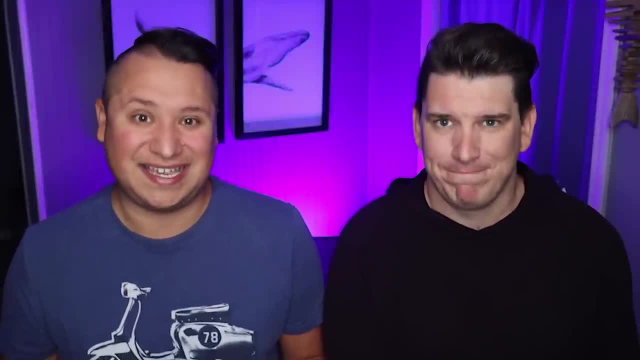 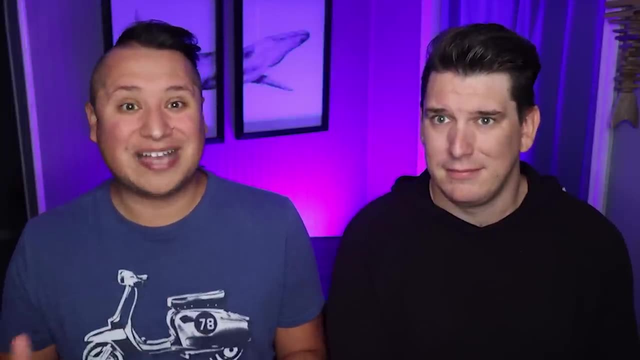 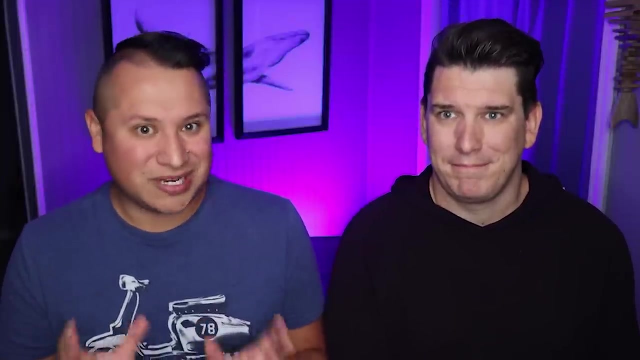 of the EU, you will have this value-added tax, the VAT, On top of that. if you have an itinerary that has one non-EU port, you will actually be able to not pay that, Unless if you're porting near Spain or out of Spain. When you're near Spain, you will always pay. 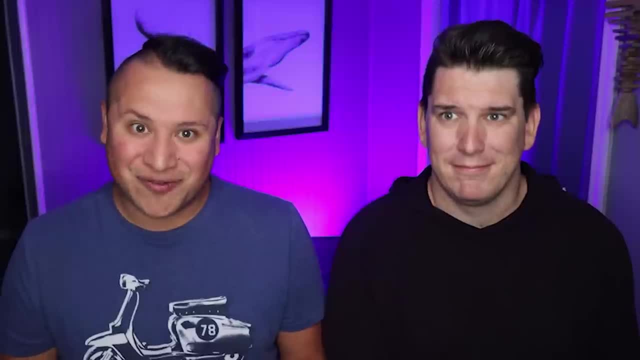 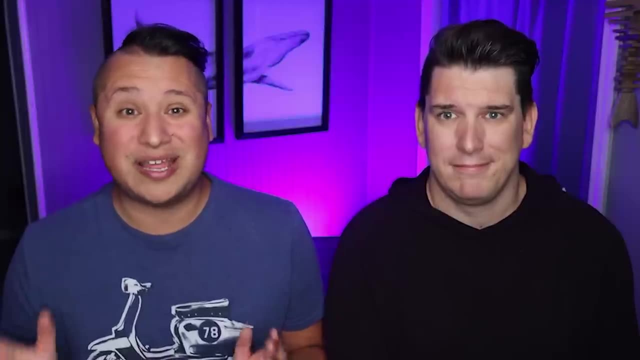 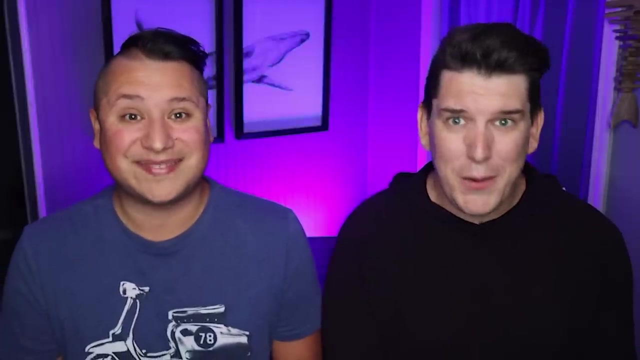 this VAT tax. However, it's something you just need to know about, because it is truly an additional cost to anything and everything onboard, including some things that you wouldn't think of normally if you're sailing out of another destination, such as North America, To give you a very practical example of this. when we got onboard, we were going to upgrade our drink packages from classic to premium. Now in the Caribbean that cost $10 per person per day plus gratuities. When we got up to the guest services desk to do this, they told us that between the heightened cost for the Mediterranean cruise and the Spanish VAT, it would be $20 per day per person plus gratuities. That is double the cost. We had no idea that that was going to be the situation and we absolutely did not upgrade our drink packages because it was double the price that we had. 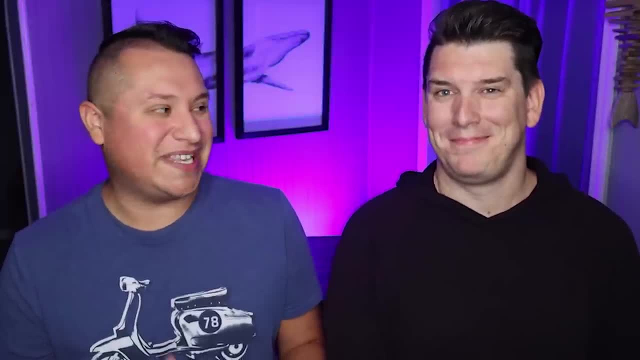 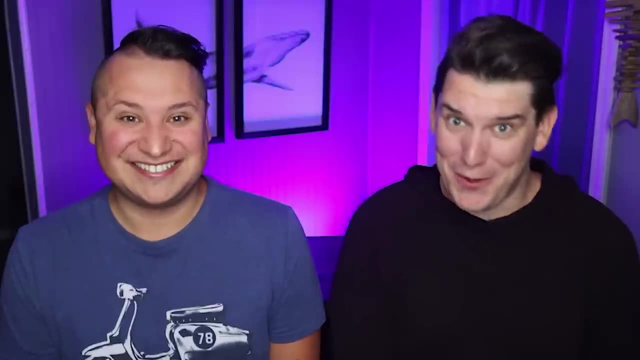 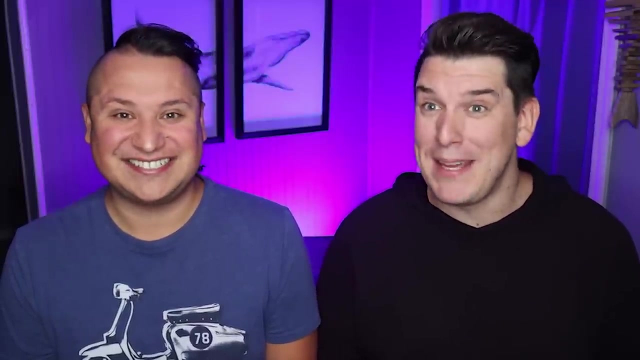 That was the end of the bad, but now it's time for our ugly, And this was truly, truly ugly, And this will change our plans in the future for any Mediterranean cruises that we ever do. Now, we said that we cruised on the Celebrity Beyond. We. 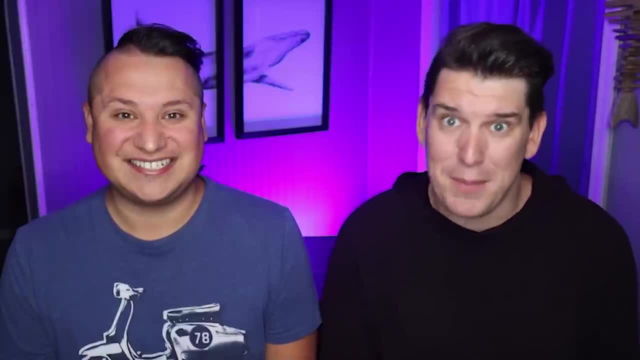 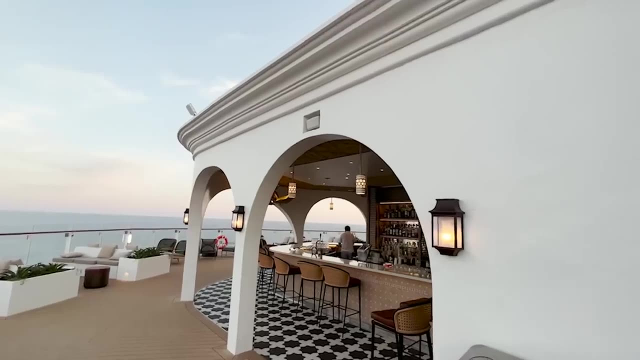 were actually on the second sailing for the Beyond. If you don't know much about that ship, you can check out our other content about that ship. We were so excited to be on this ship because we love that class of ship. We love that class of ship, We love that class of ship. 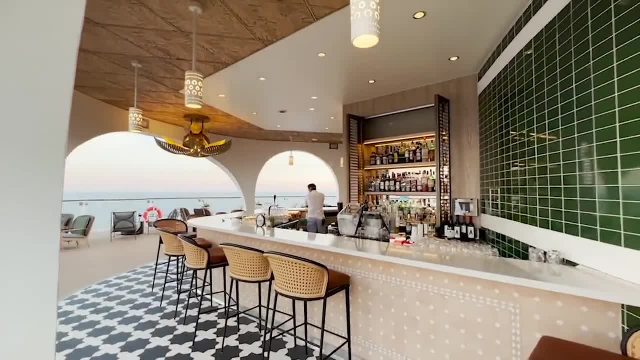 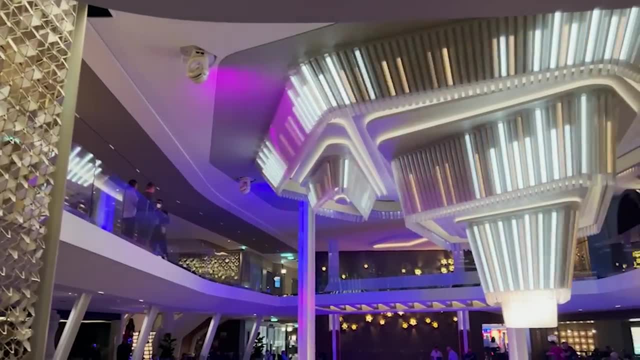 This was probably the most anticipated ship of 2022 for Jared and I, and we just could not get on the ship fast enough and experience and enjoy everything the ship had to offer. Unfortunately, with Mediterranean cruises, if you haven't gotten a gist based 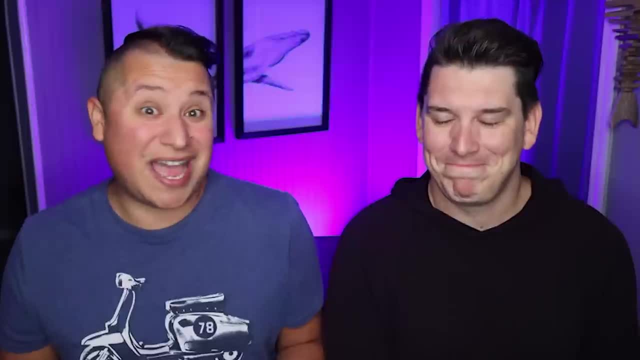 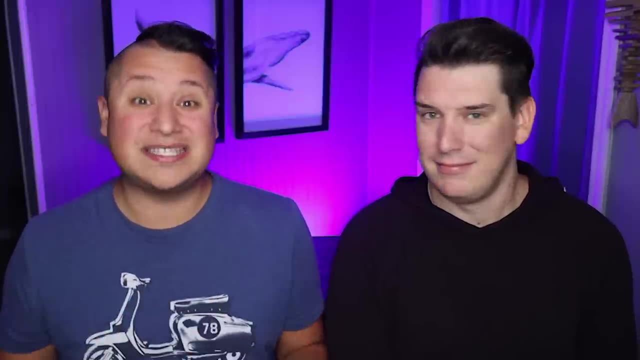 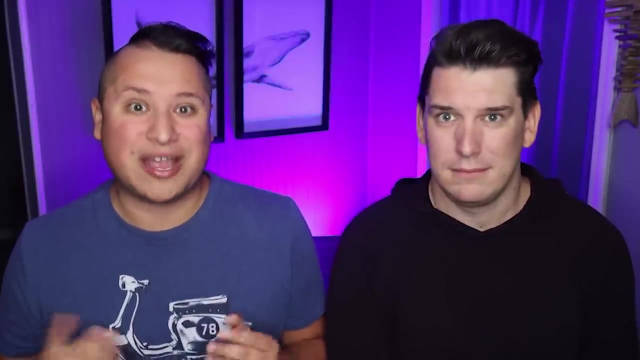 on everything we said in the bad. you don't spend much time on board your cruise ship. In fact, for Mediterranean cruises, the time on board your ship is the least amount of time we have ever spent on cruise ever, and that is probably by a good average of three or four more extra hours a day. 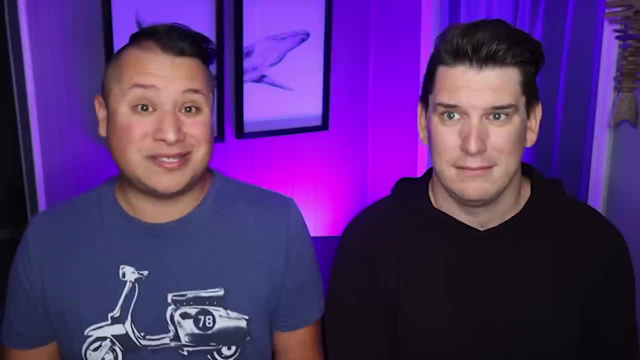 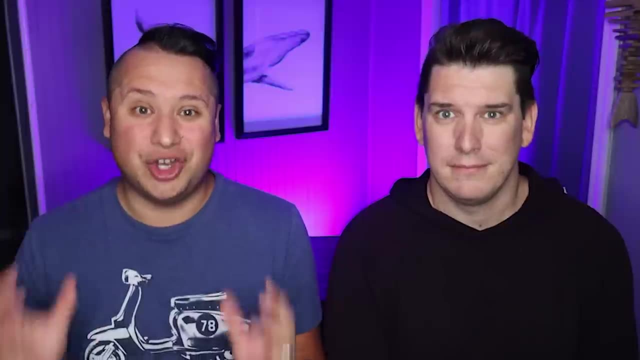 that we did not spend on board. You're at port, You're experiencing all these new destinations, but when you pay a really good amount of money to be on one of the best newest cruise ships of the year, you want to be on board and experience all the shows, entertainment. 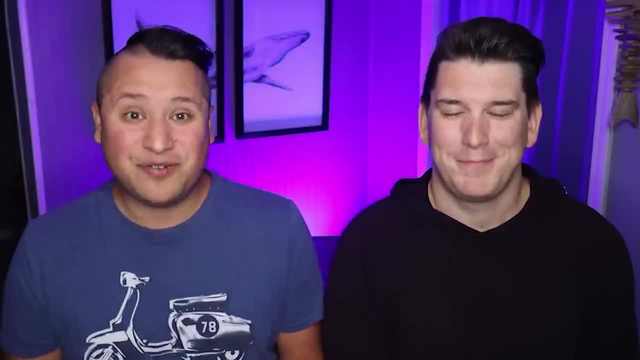 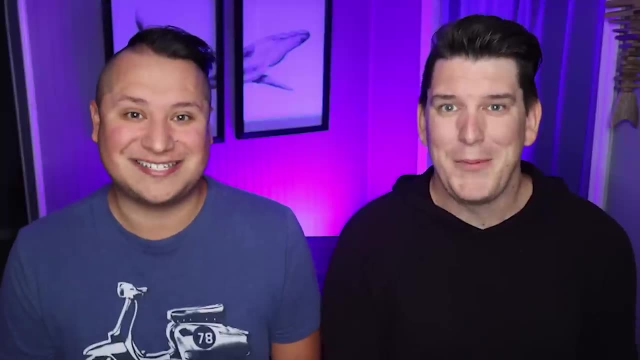 the amazing food and beverages and service that you paid for And unfortunately, for Mediterranean cruises. the time on board your cruise ship is the least amount of time that we have ever spent on board. You don't experience that nearly enough to pay that cost. We know a lot of you at home. 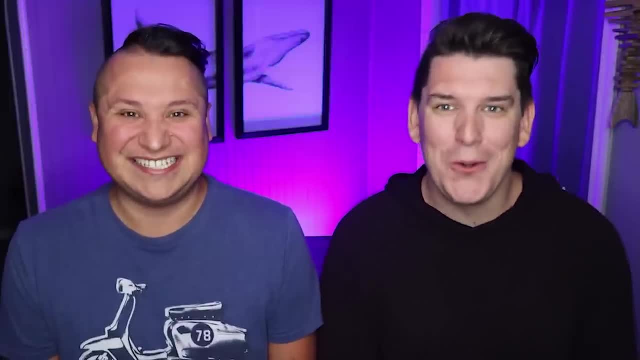 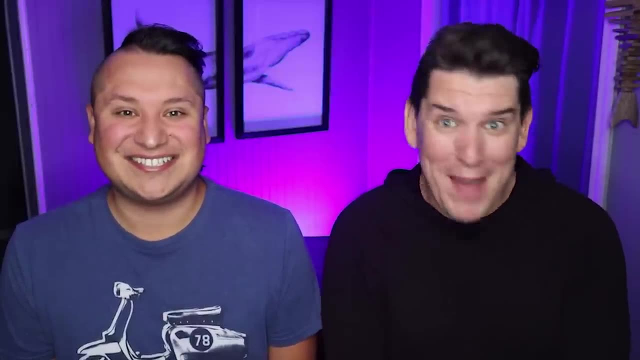 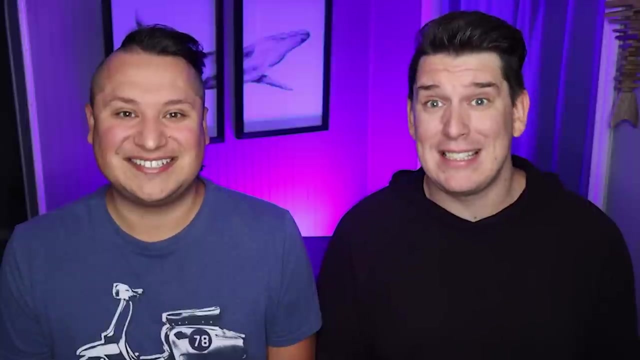 are cruise addicts and love cruising and for many of you, the ship is the destination. So this is our ugly: Do not make the ship the destination. when you are cruising in the Mediterranean, The ports should be the destination, The countries that you're. 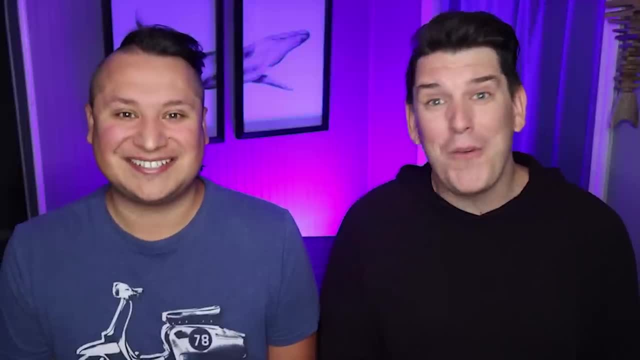 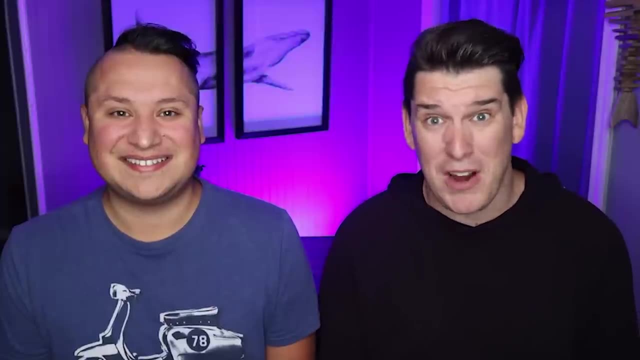 visiting should be the ultimate goal. If you're coming over to the Mediterranean and spending all the money to fly over here and take a Mediterranean cruise, you need to know that you're not going to be on the ship very much and that, while the ship might be wonderful and lovely, you're probably not. 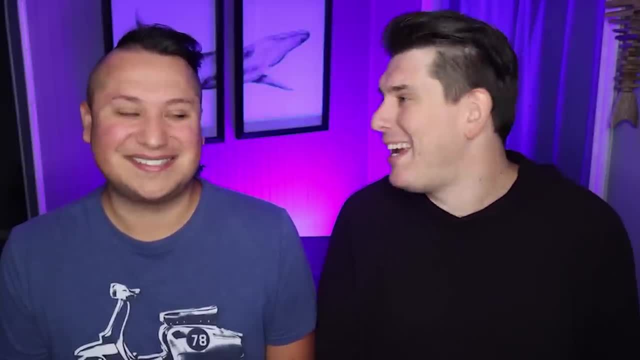 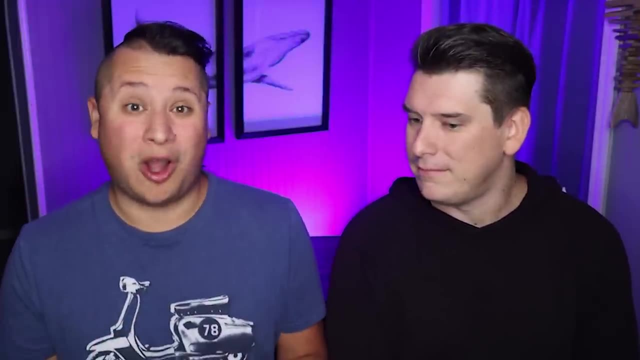 going to get to experience it and enjoy it in the way that you would, let's say, in the Caribbean or other parts of the world? Yeah, and of course I want to mention this- The perspective is different depending on who you are. We know that we have viewers from around the world. If you are somebody, 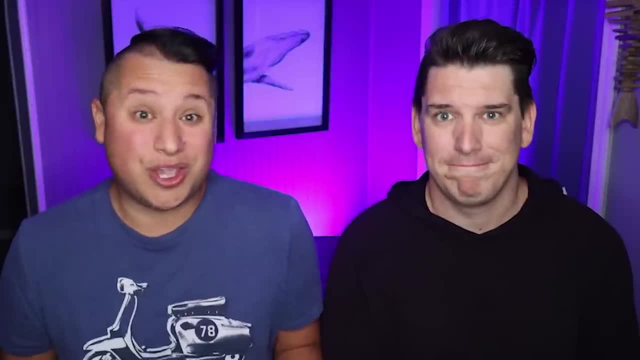 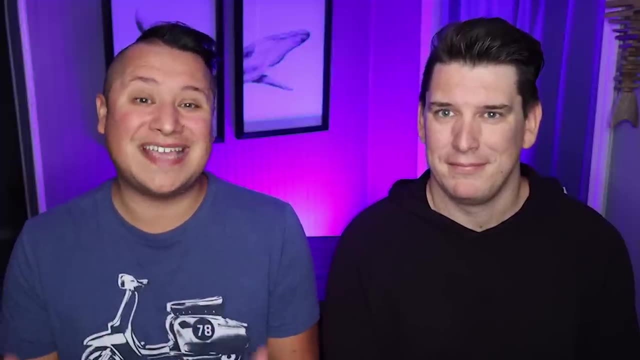 that is living in the European Union right now. this may be your Caribbean. This may be the time where you do visit every port that you've already been to many times, and if that's the case, that's awesome. Pick it, Pick the best ship possible so you can enjoy while on board, because a lot of other people 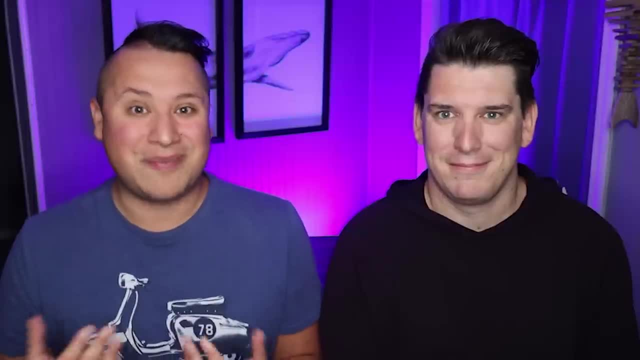 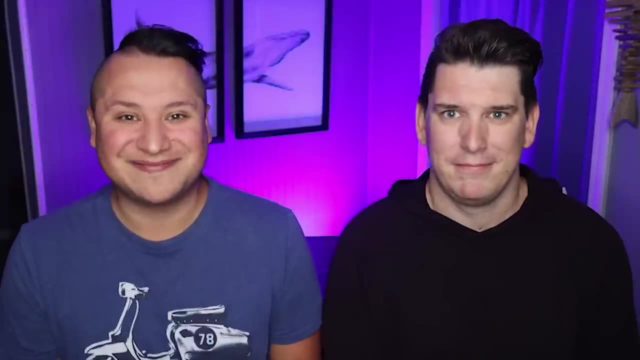 are going to be at port, but for those like us in the North American region or that aren't in Europe or the EU experience the ports. Those are your destination, just like Jordan said. Well, thank you so much for watching. We want to hear from you. Have you taken a Mediterranean? 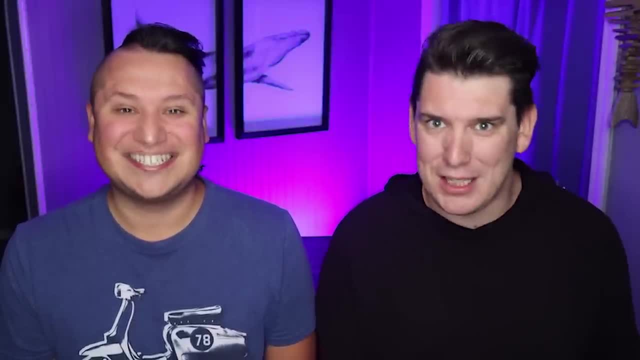 cruise and, if so, were these tips helpful? Do you have additional tips? We've been doing this in our comments lately and I really like it. We're letting the comments be a resource for people. so if you have additional tips to share about Mediterranean cruises, if you feel like you've- 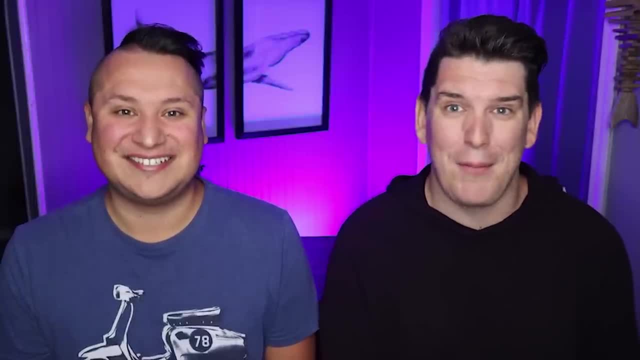 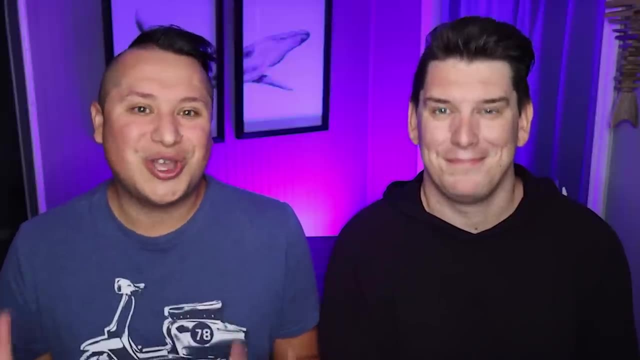 learned something that we didn't share today. please drop it in the comments below, And, of course, this is just our experience. If this is different for you, we want to hear that because we want to give as much good feedback and information for people planning their next Mediterranean cruise. 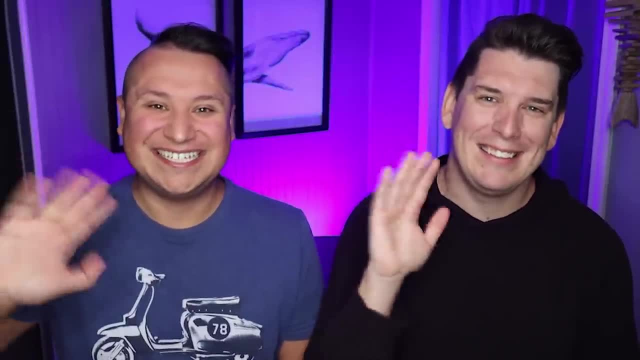 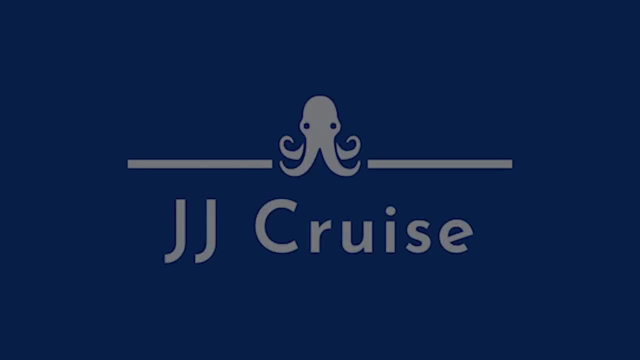 Thank you so much for watching and until next time. see ya, Jake Bruce.